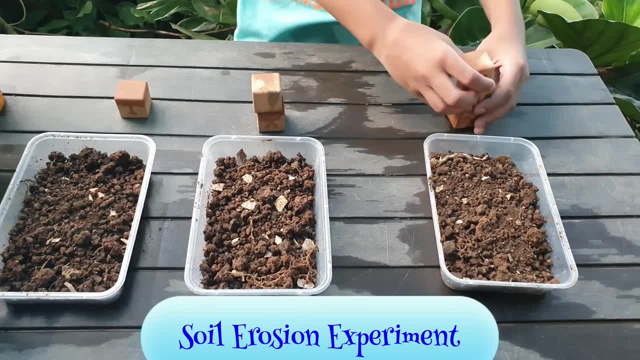 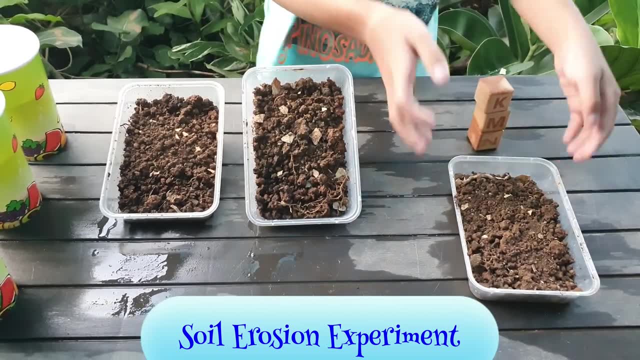 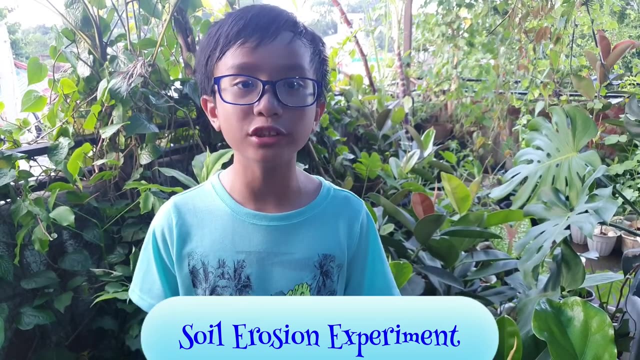 of soil. we will use three blocks underneath. Now let's put this on top. And now time for the second tray. And now the third tray. Let us see what will happen if we pour water in each tray of soil. So here's the first. 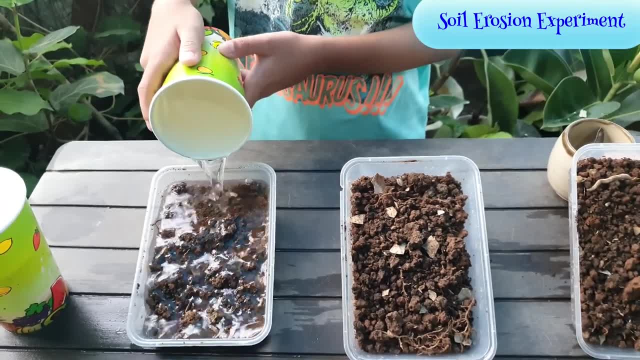 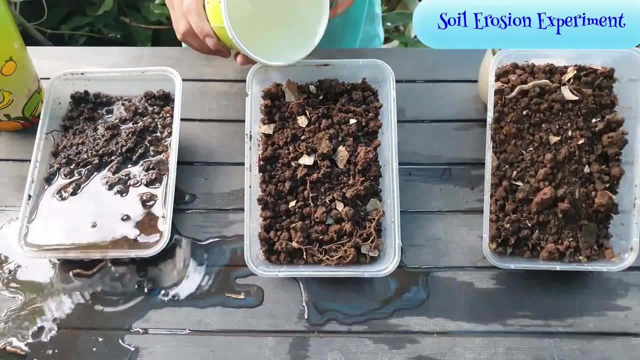 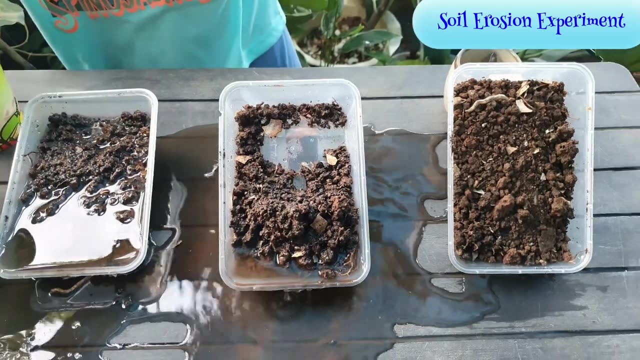 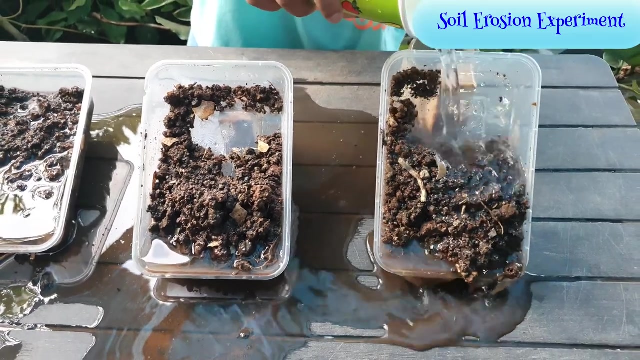 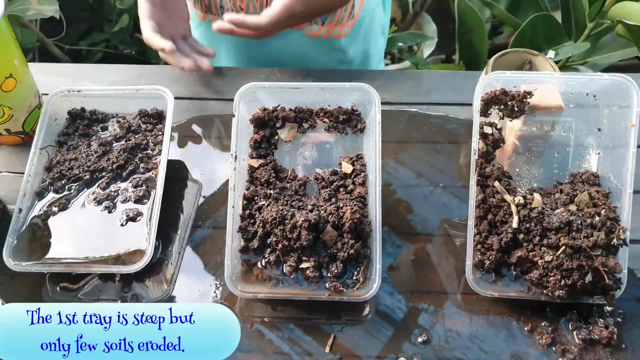 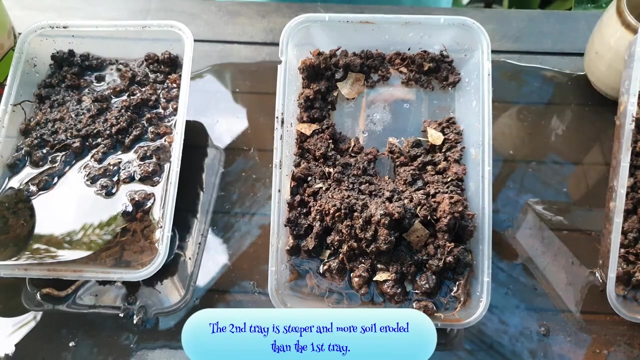 tray filled with water. And now the second tray, And now, last but not least, the third. We observe that the first tray is steep, but only few soils eroded. The second tray is steeper and more soils eroded than the first tray. The third tray is the steepest. 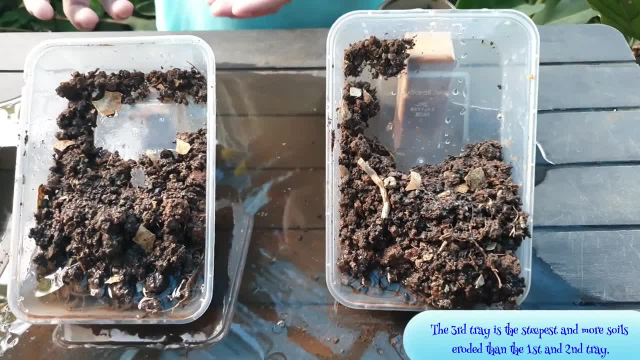 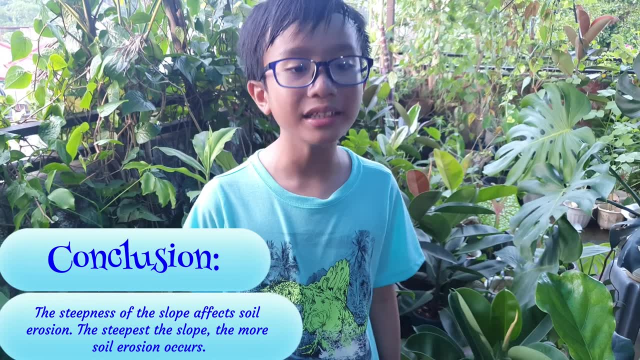 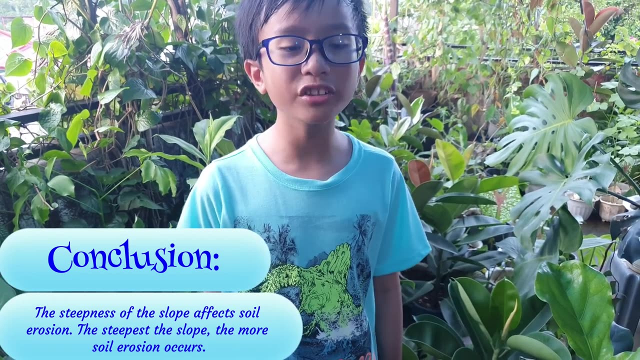 and more soils eroded than the first and second tray. See, it is more tilted than the first, The other tray. I therefore conclude that the steepness of the slope affects soil erosion. The steepest the slope, the more soils erosion occurs. 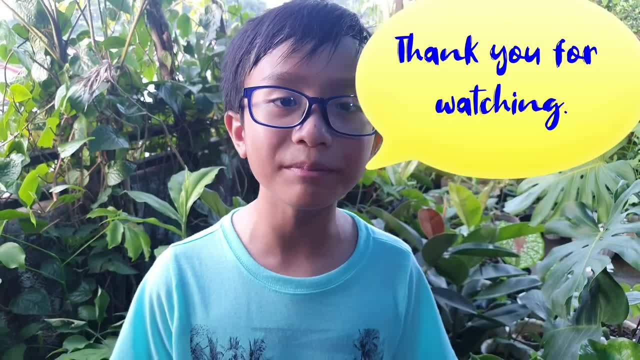 Thank you for watching this video. I hope that you learned something from this video. Byeötttttt. 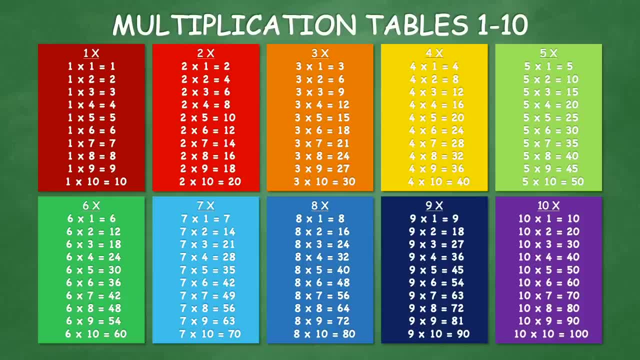 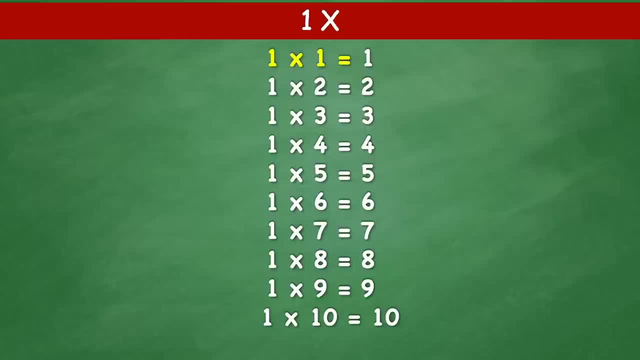 Abacada Multiplication Tables 1 to 10: 1 x 1 x 1 equal 1. 1 x 2 equal 2. 1 x 3 equal 3. 1 x 4 equal 4. 1 x 5 equal 5. 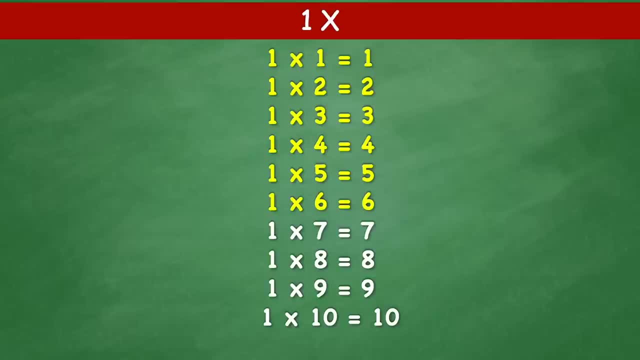 1 x 6 equal 6. 1 x 7 equal 7. 1 x 8 equal 8. 1 x 9 equal 9. 1 x 10 equal 10. 2 x 2 x 1 equal 2.